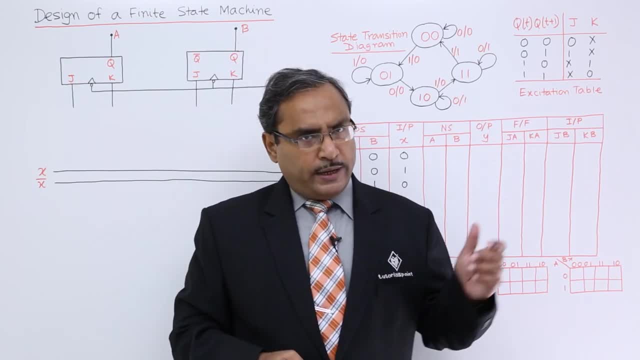 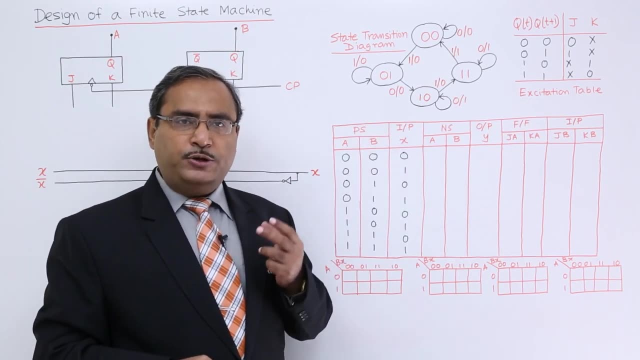 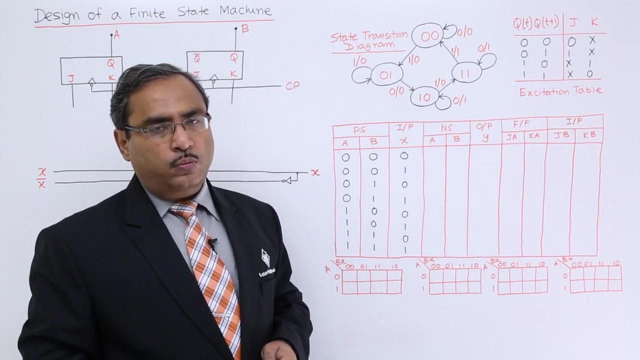 Design of a finite state machine. So here is the state transition diagram of the machine given to us. It is having four states, So that is why two bits will be just enough to represent the state numbers. So 00,, 01,, 10 and 11.. Now how to read this finite state machine. So for 00 state. 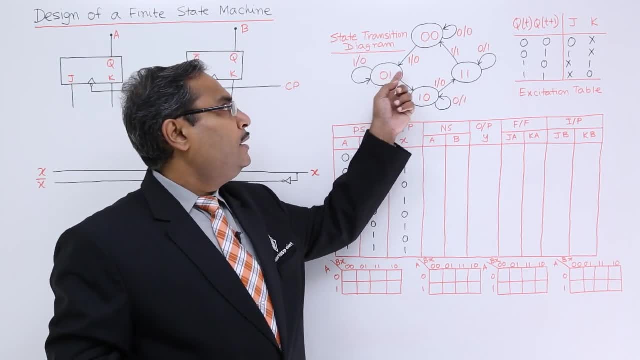 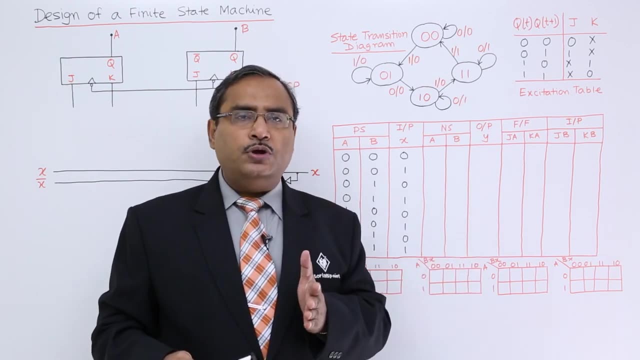 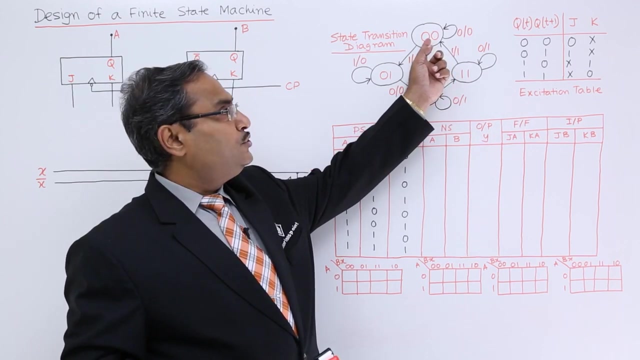 if I provide the input 1,, then the next state will be 01 and output will be 0. So it is denoting input and it is denoting output, As we say input output. so it has been written as input slash output. So in this way you can also mention that for the state 00, if I provide the input 0,. 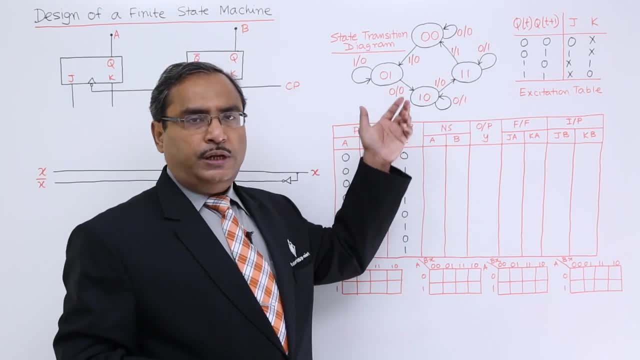 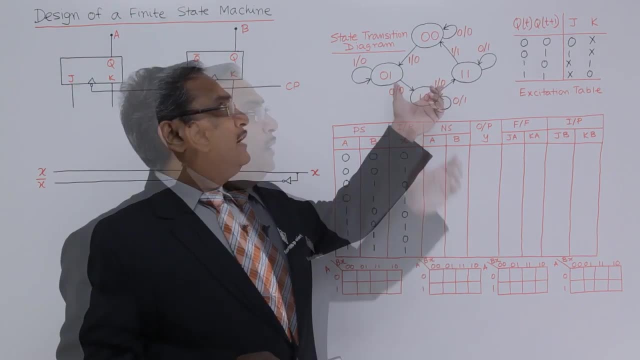 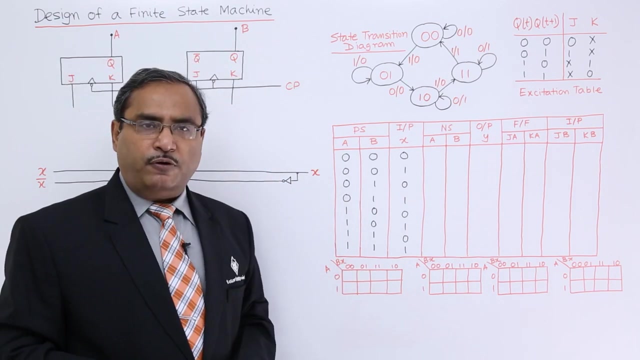 then the output will be 0 again. So this machine is given to us and we are supposed to implement it in our sequential diagram. So how to implement it? At first we shall map this respective state transition diagram onto this table. So here is the table for us. So now let me go for the fill up of this columns. So 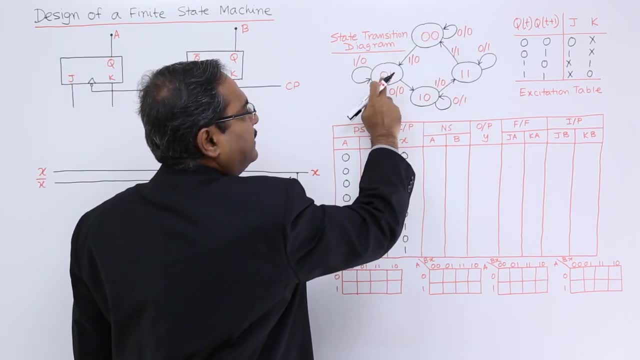 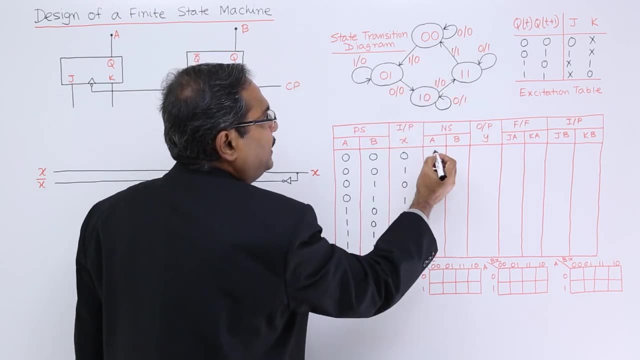 for a- b. so that means a is this one, this is b, a, b. in this way we are writing. So for 0, 0 state for the 0 input next state will be our next state will be our 0, 0 and output. 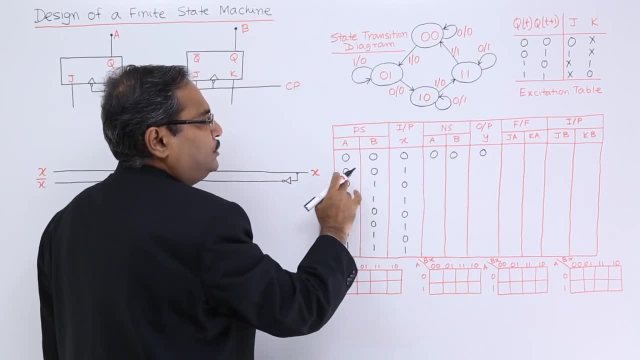 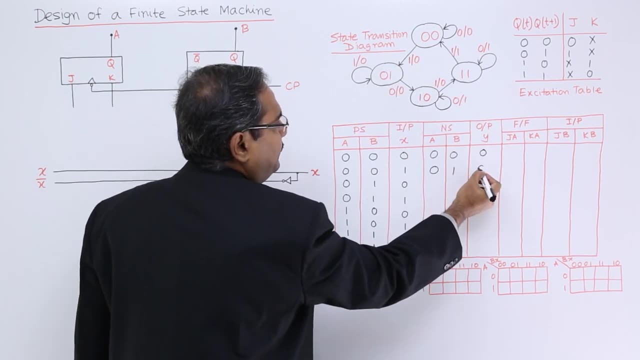 will be 0 here. So in this way we shall fill up for 0, 0 state for 1, input. we are finding the next state will be 0, 1 and output will be 0 here. So in this way we are going to. 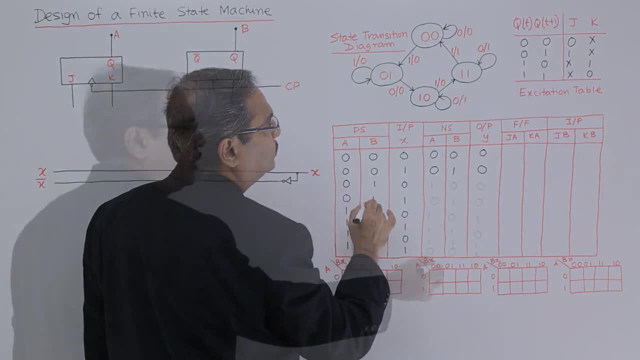 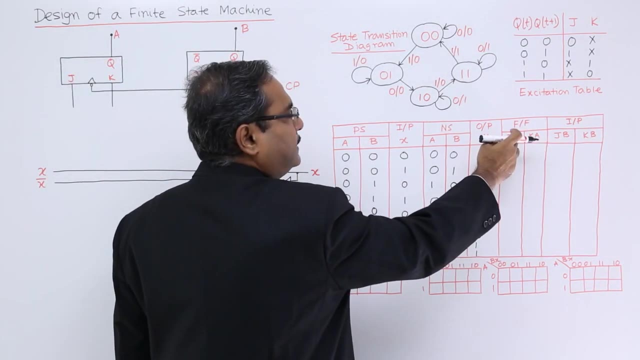 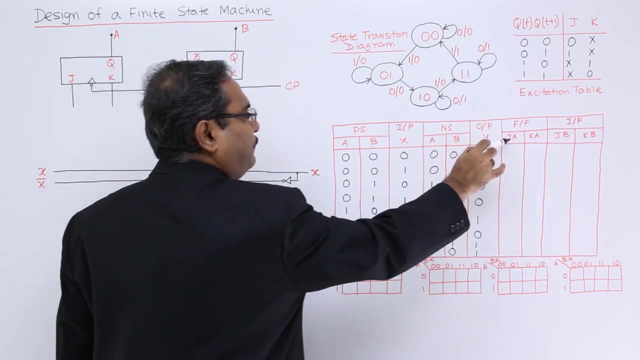 fill up this respective table. So we have completed this rest part of this columns. Now we are going for this j a, k a and j b k b column fill up. So here we shall consider this a and a column to fill up this j a and k a. Here we are having the excitation table. 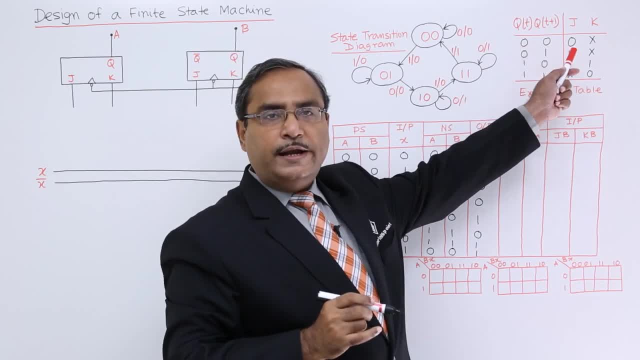 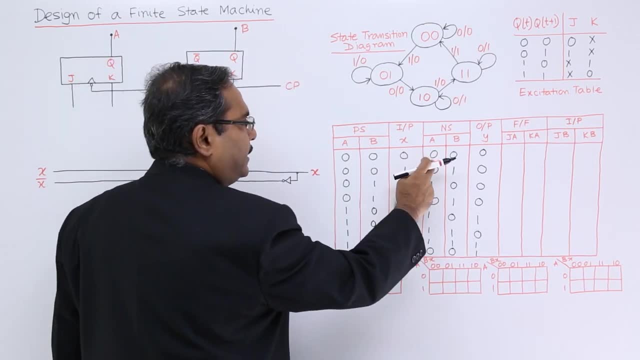 of j, k flip flop. So form for 0 to 0 transition I require j and k should be 0, x. in this way we have written it. So now we shall consider a and a column here. that is a present state. 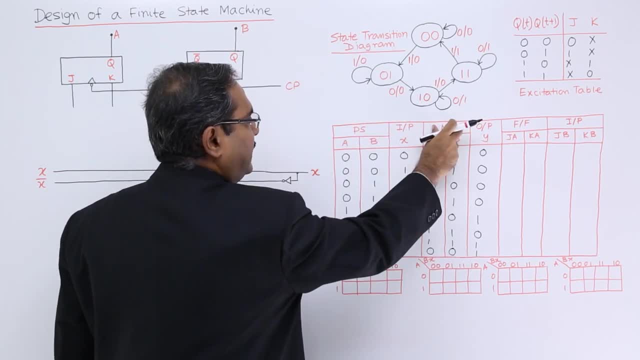 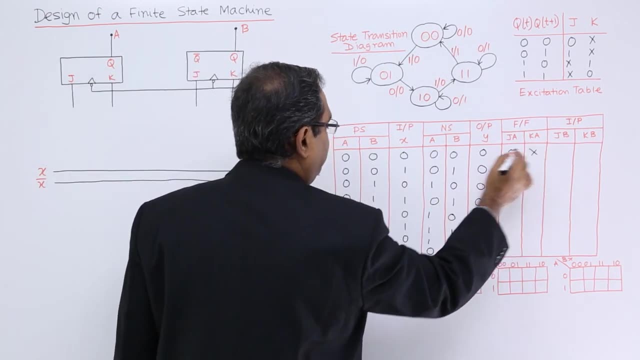 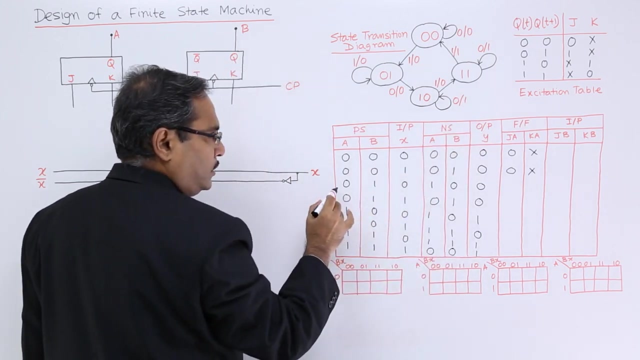 and the next state. So p? s stands for present state, n s stands for next state. accordingly, we shall fill up this j, a and k a, So 0 to 0 transition. we are writing this one as 0 x, So 0 to 0 transition. we are writing this one as 0- x. as it has been mentioned, 0 to 0. 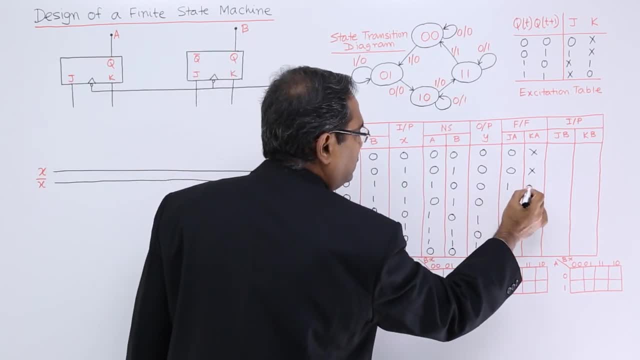 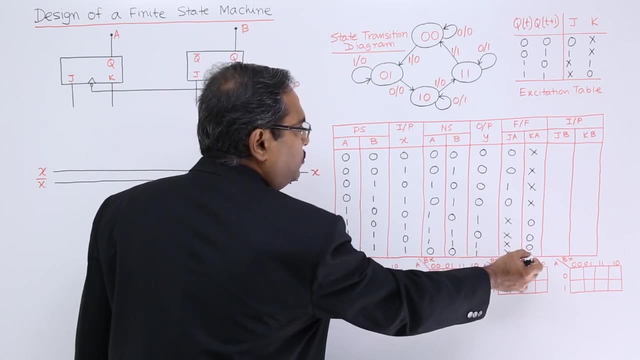 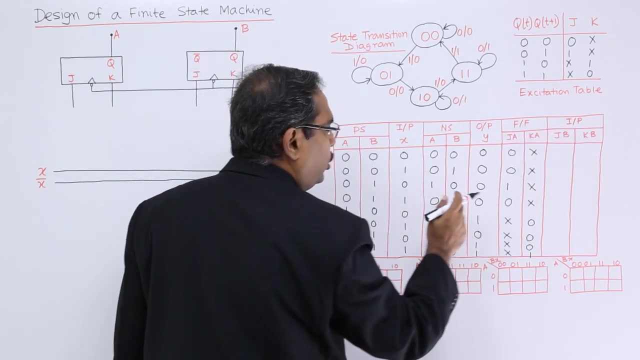 to 1 transition. we are writing this one as 1 x. in this way we are filling up the rest. Now we shall go for the b columns, for the present state and the next state, and accordingly j b k b will be filled up. So we are writing the respective j b k b values considering: 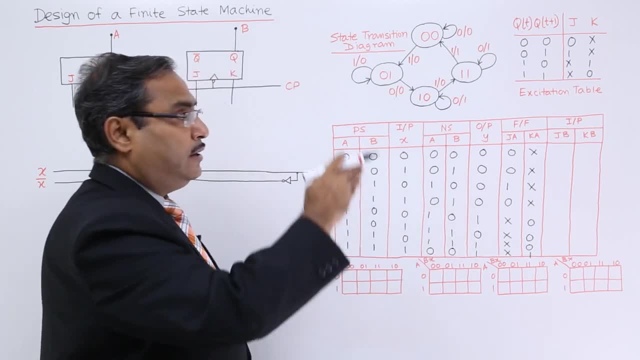 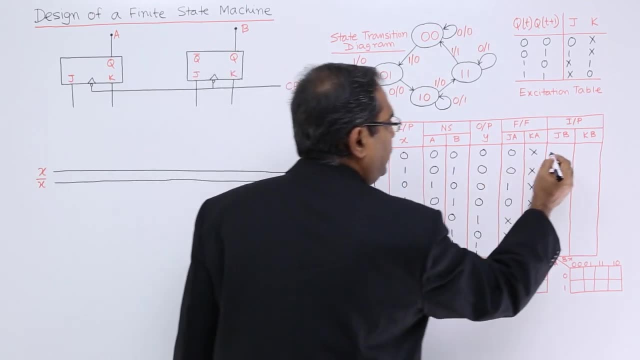 b column for the present state as well as for the next date, and we shall take the help of the excitation table. So here we have the j a, k a. we are working on this- j a and So 0 to 0 transition. 0 to 0 transition. we require this one as 0 x, as it was mentioned. 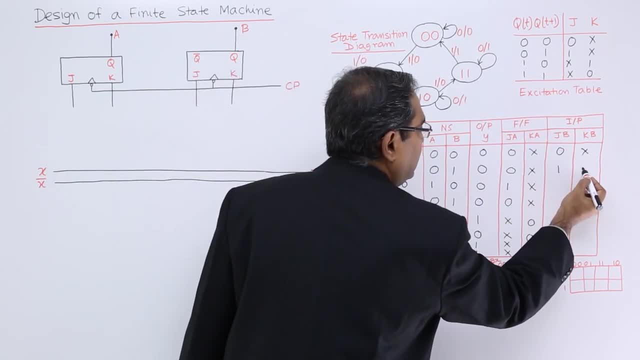 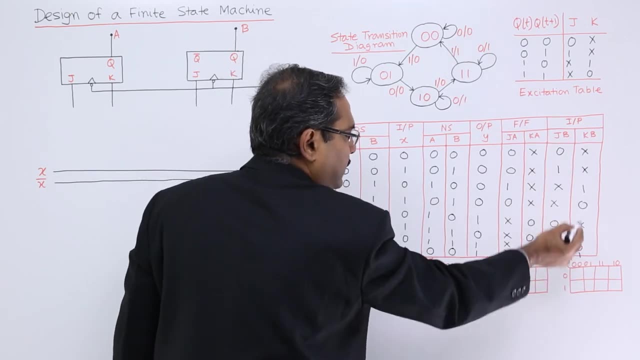 So 0 to 1, we are going for 1 x. In this way we are filling up the rest Now. in this way, we have filled up this j, b and k b columns. Now we shall have to find out the Boolean. 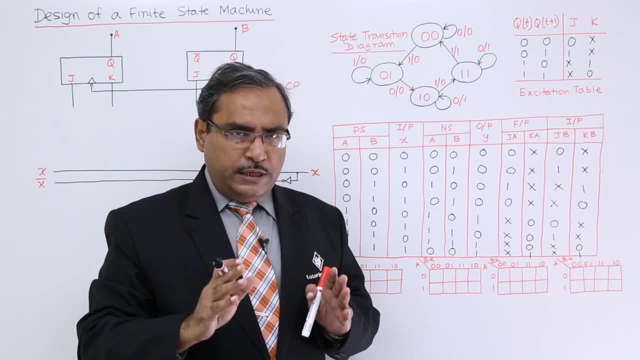 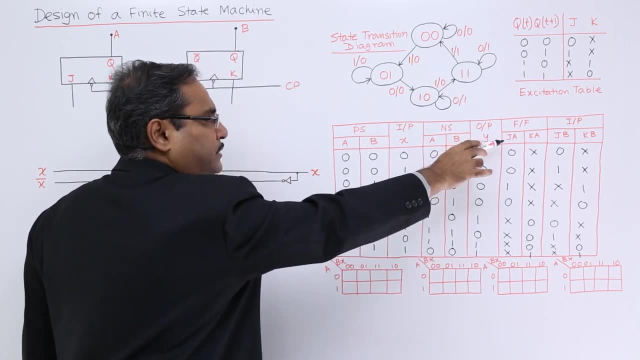 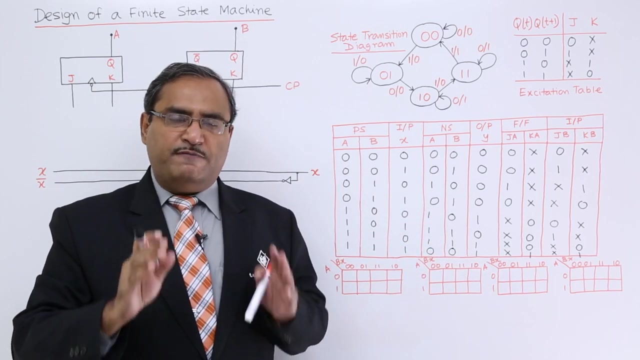 expressions for j a, k a, j b and k b and also for the output. So now let us consider the j a at first. We shall be plotting this j a against this a, b and x in our kernel maps If we do not get the respective Boolean function. just judging this truth table. So 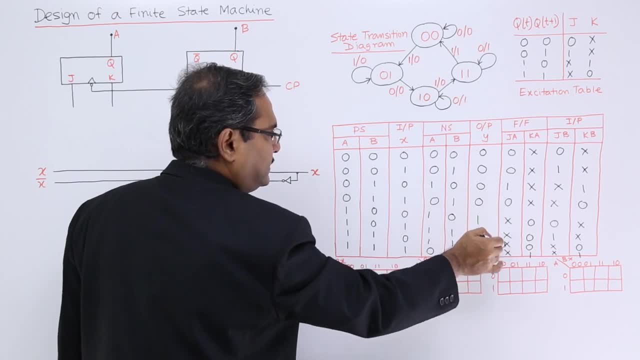 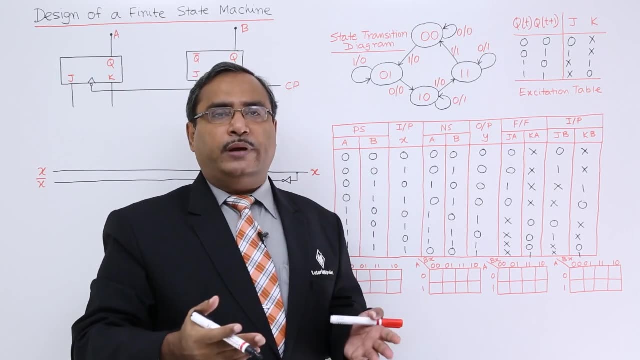 here we are having this: 0, 0,, 1, 0, x, x, x, x. So now, from here it is not possible to get. So that is why you can go for the kernel map. Otherwise, if you can get the Boolean. 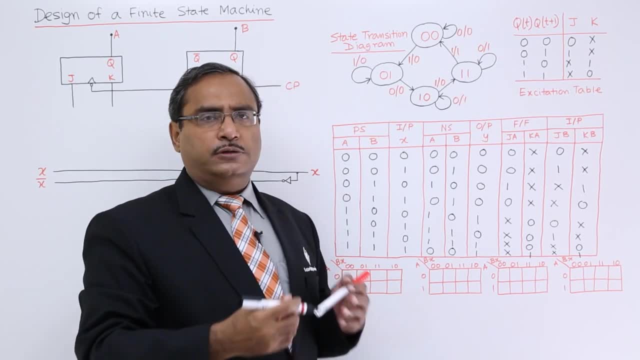 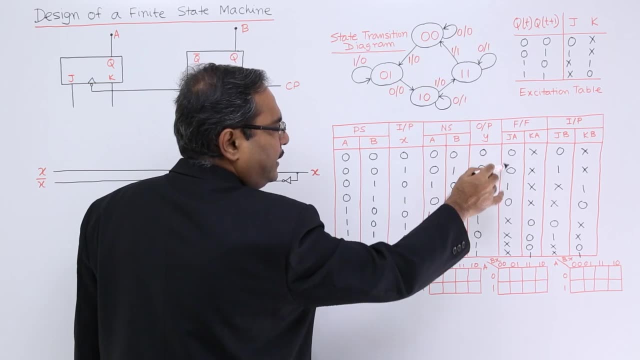 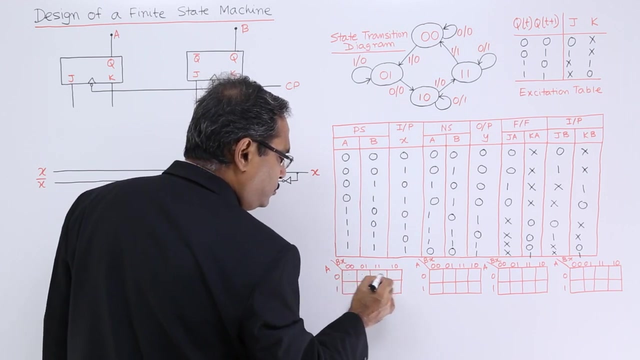 function directly. you can omit the kernel map steps. that will save your time while answering this question. You can write the Boolean function directly. So now we are going for this. j a plotting 0, 0,, 1, 0, x, x, x, x. I am plotting here. So 0, 0, 1, 0, x, x, x, x. So here. 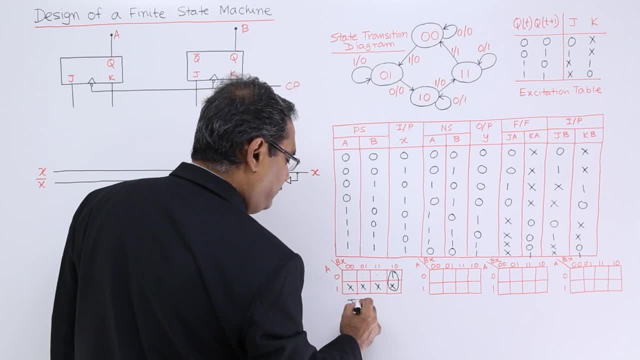 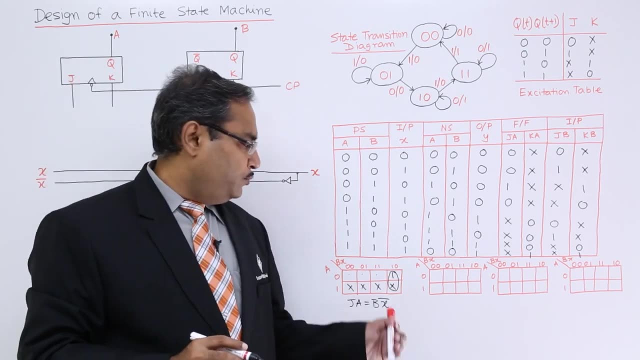 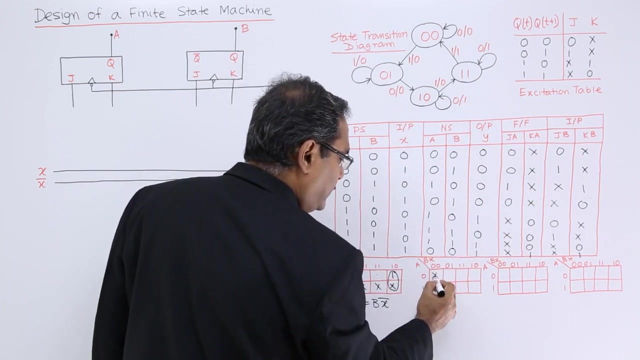 the covering will be like this: So I shall be going for j a, which is nothing but b x bar. So j a will be b x bar. we have written. Now we shall go for k a, So k a. here we are having x, x, x, x, then 0,. 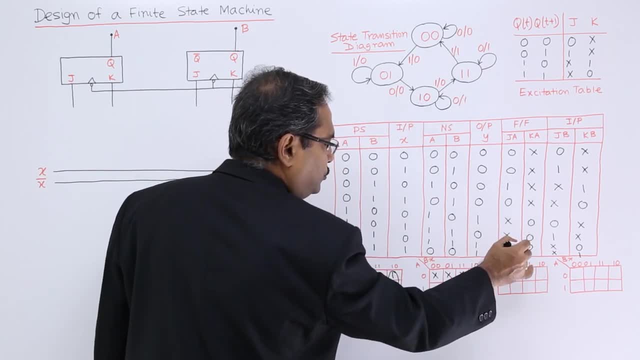 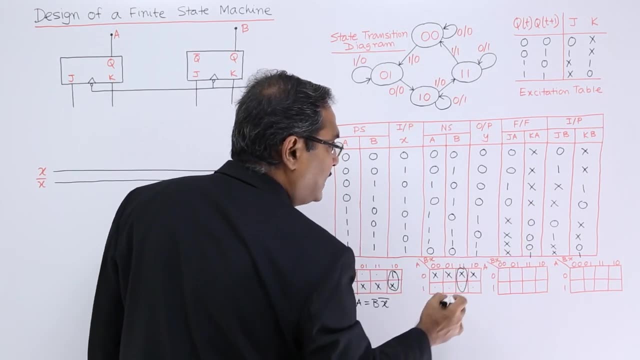 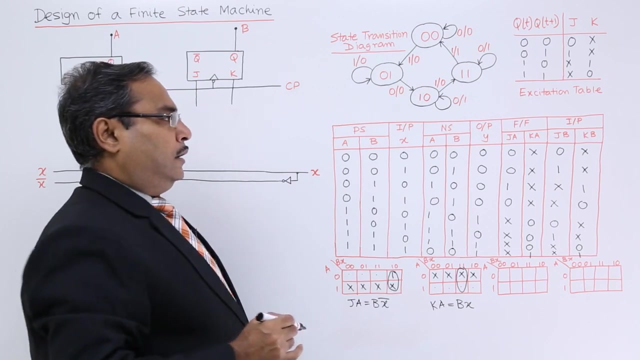 0, 0, 1.. So if we do the covering here, we are going to get this k a as 0, 0, 0, 1, x, x, x, b, x. Now we shall go for the j b. now We shall go for the j b. j b is having. 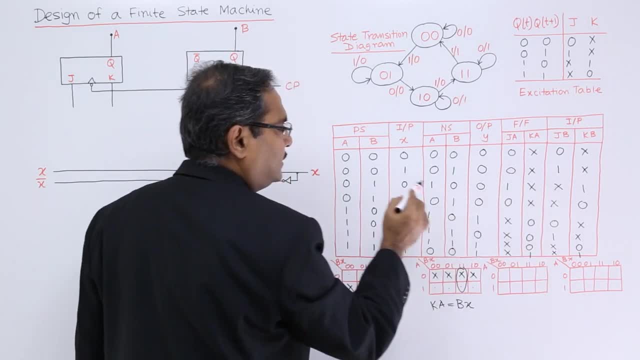 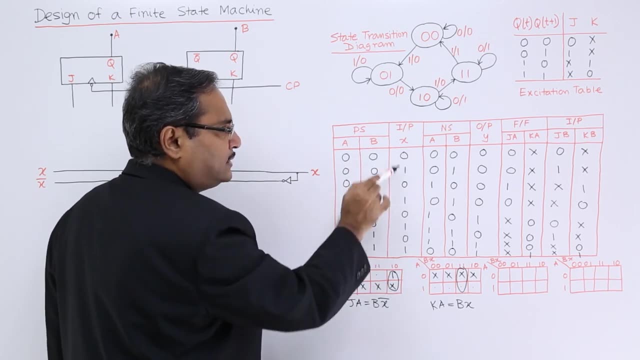 our 0, 1, x x. 0, 1, x, x. So we are finding this one as 0, 1.. We are having this x means anything, 0, 1.. So we are matching with this x here. We are matching with this x, So j. 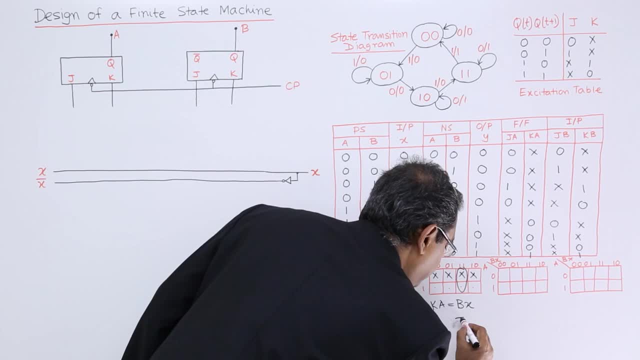 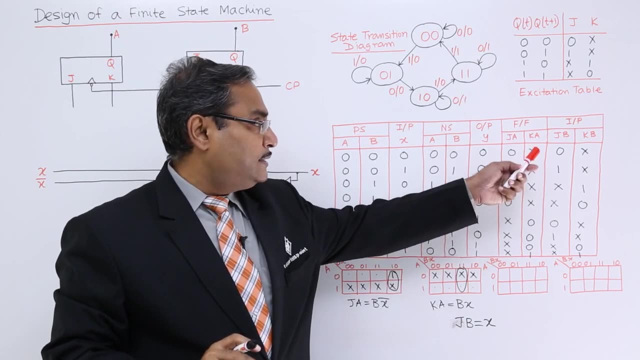 b for j b. I am writing this one as x here. So j b for j b. I am writing this one as 0, 1.. Now we shall go for this k b. So x, x, 1, 0, x, x, 0, 1.. So x x, 1, 0, x. 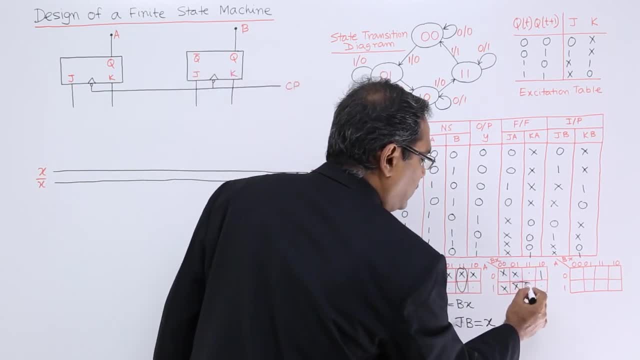 x, 0, 1.. So here is the covering for us, and another cover will be like this. So we shall go for this one as k b. So it is a bar, it is a bar, and here this last 0 is coming. So 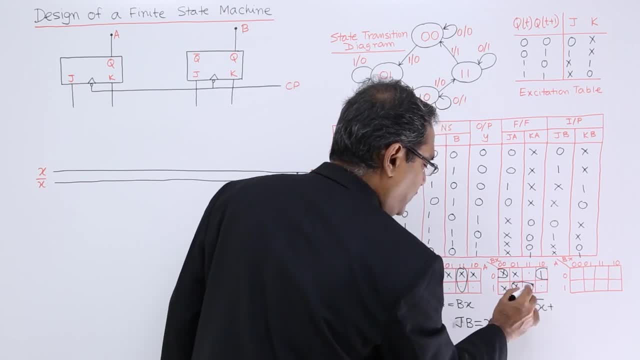 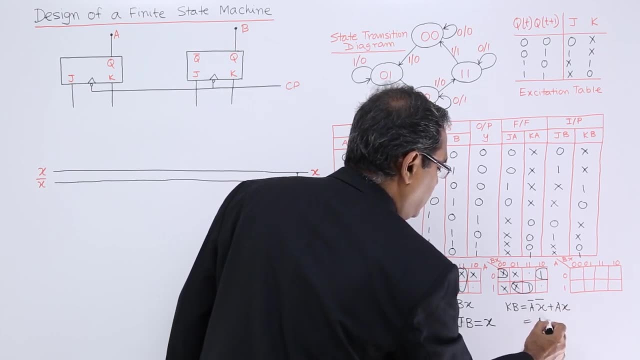 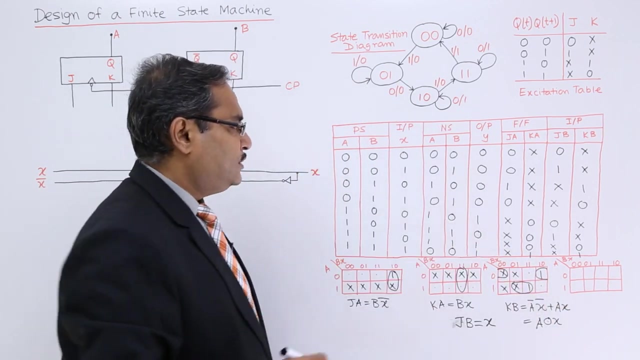 it is a common x bar plus this one is a, and here this x is common, So it is a in zone x. Let us go for the y also. y is remaining, So y is this one: 0, 0, 0, 0.. We are having. 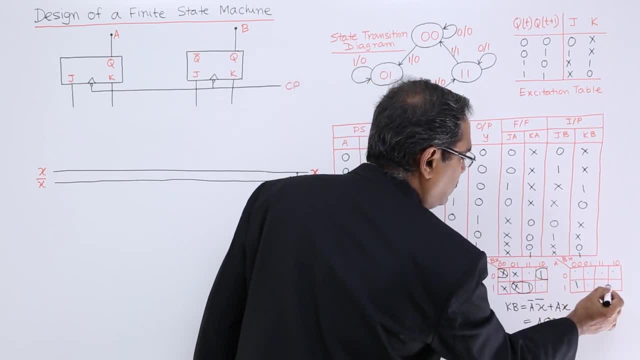 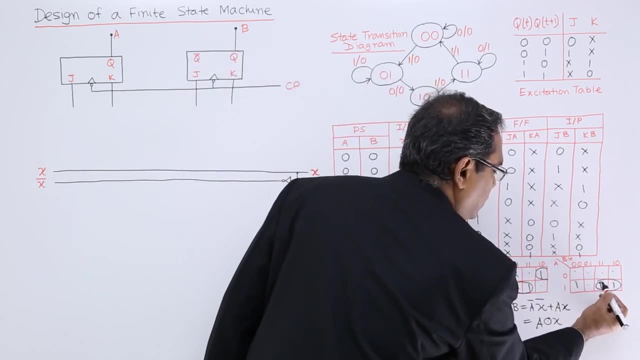 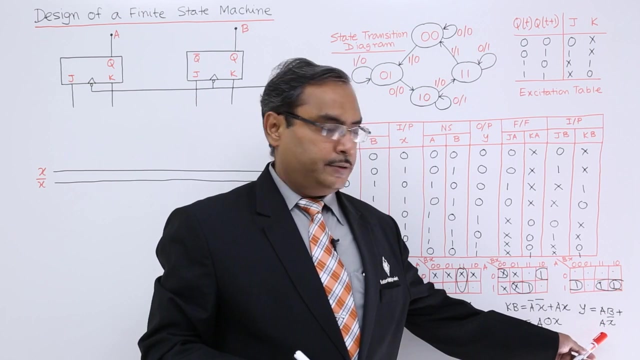 this one, this one: 1, 0, 1, 1.. So we are having this. So now we are having two covers and another cover is like this: So in this way we have done it. So y, I have written k, b, j b, k a and j b. Now let us go for the implementation.